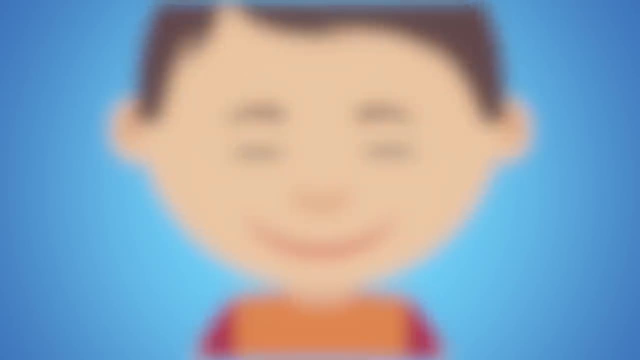 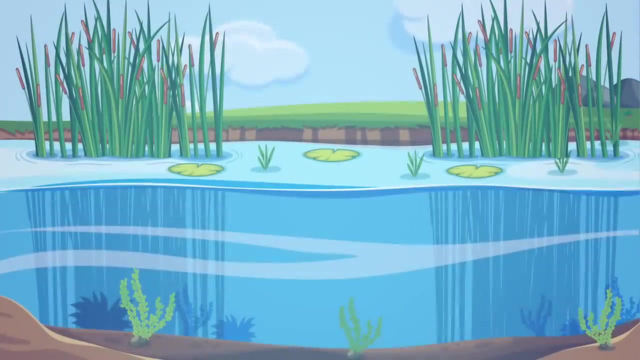 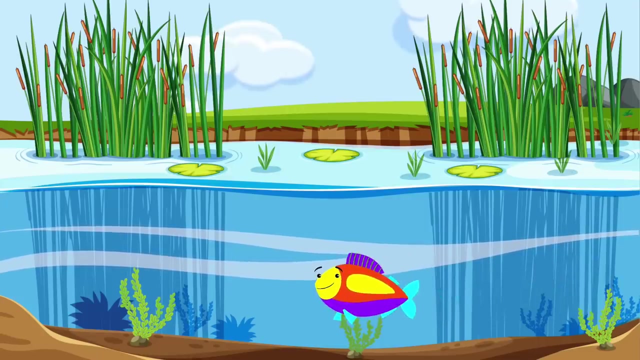 In that pond are lots of different kinds of fish- These are your feelings- All swimming around together. There's a happy fish, A sad fish, A sleepy fish, An excited fish, An angry fish, A worried fish, A playful fish. 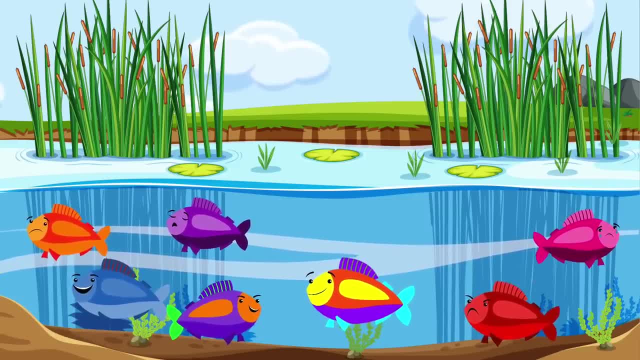 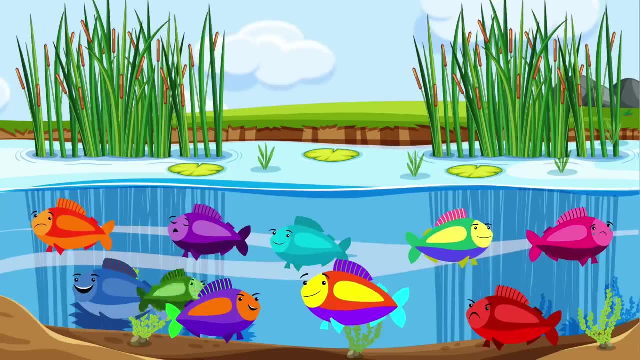 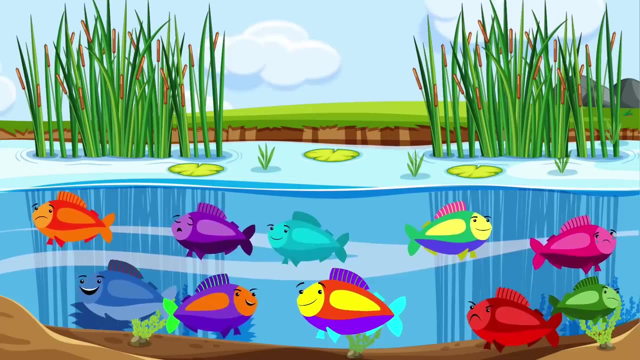 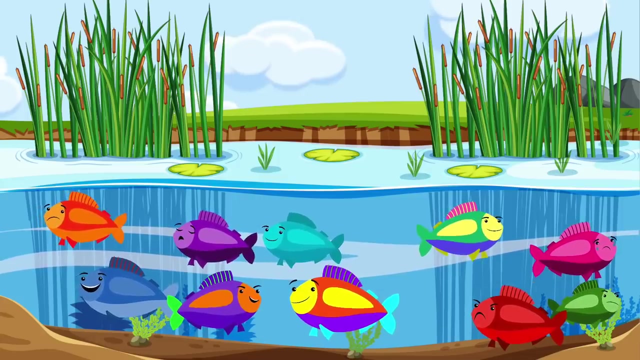 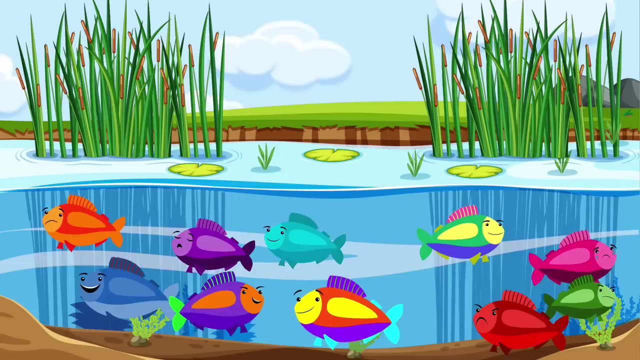 A calm fish, a kind fish, a selfish fish. so many fish, so many feelings, all swimming around the pond. Your job here is just to be the pond, Be the pond. It's wonderful being the pond, because you can just watch all your different feelings. 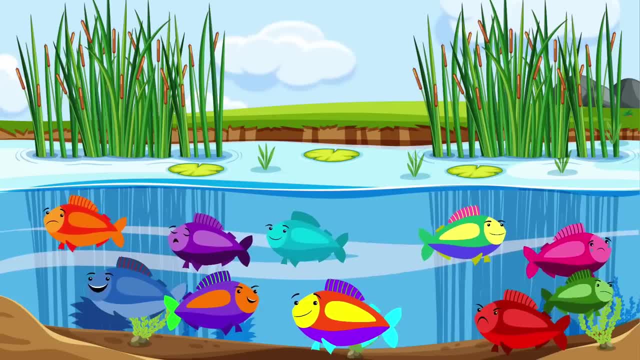 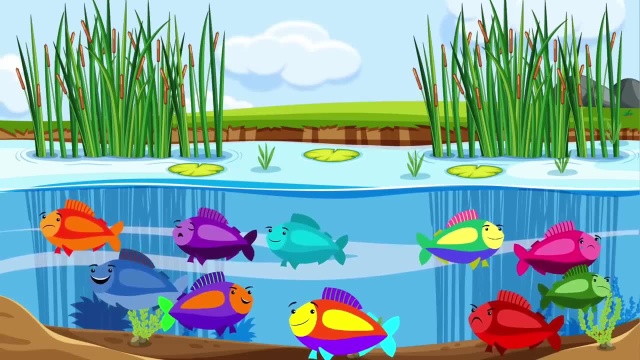 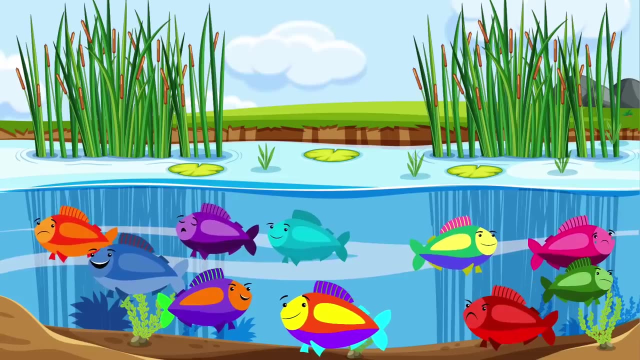 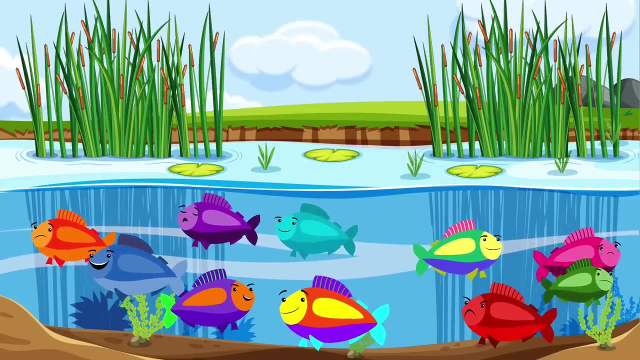 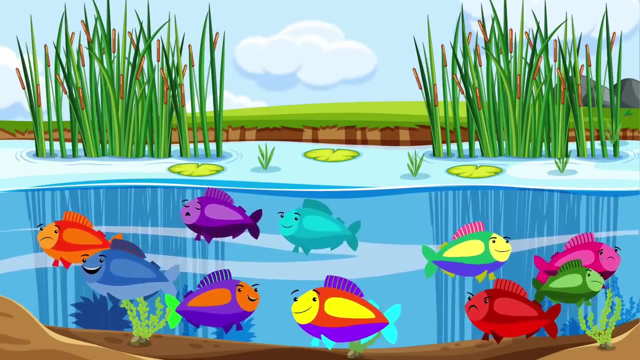 just swimming by. All of them are okay. Every feeling is welcome. You be the pond and let the fish be the fish. No need to do anything with those feelings, except watch them swimming around, See if you can be the pond. Be the pond now and just watch, seeing what kind of feelings you're feeling. 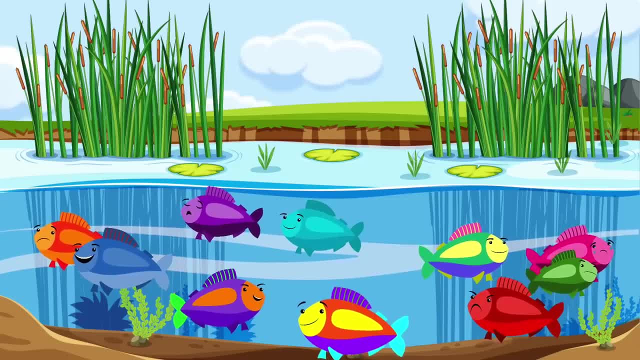 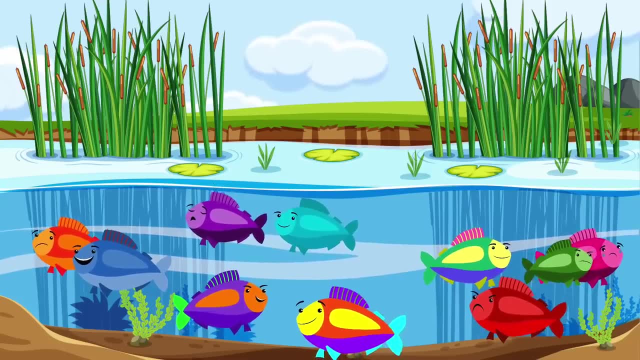 They just swim past and you can just watch them. Remember, be the pond, Just be the pond. And if we follow this special Zenden exercise, we are usually able to be the pond. And if we follow this special Zenden exercise, we are usually able to be the pond. 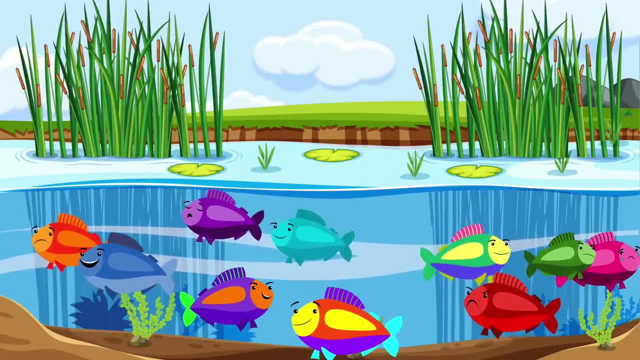 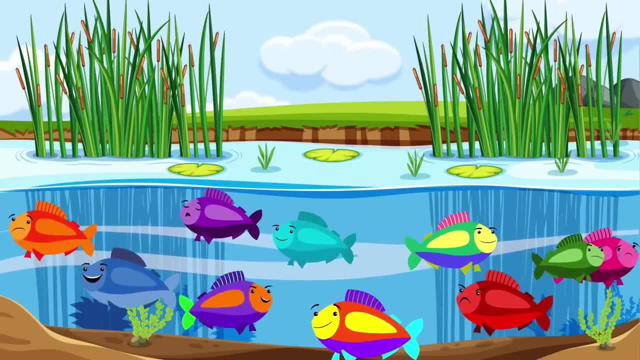 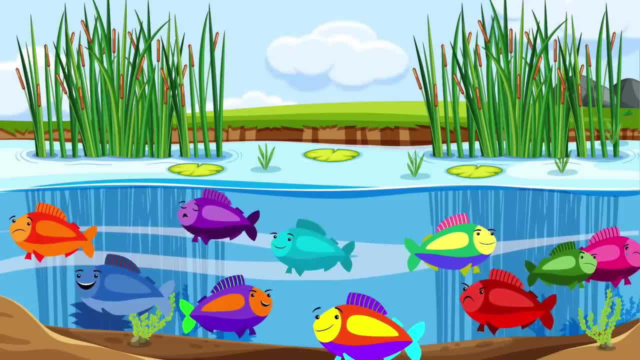 Just be the pond, Jos faz, iじゃ nod naar bạn hoặc polemical Tzie Je vì giờ mời anh Shel audible ko. we might feel like it's hard to let them just swim by. 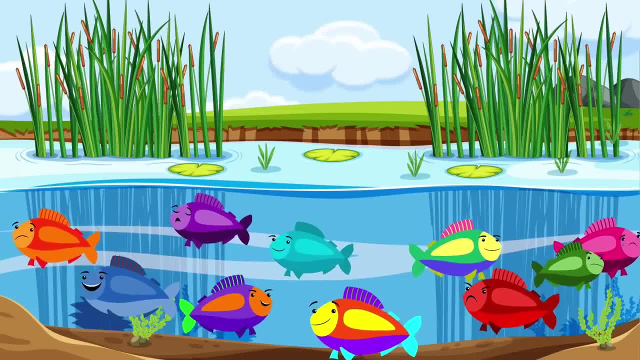 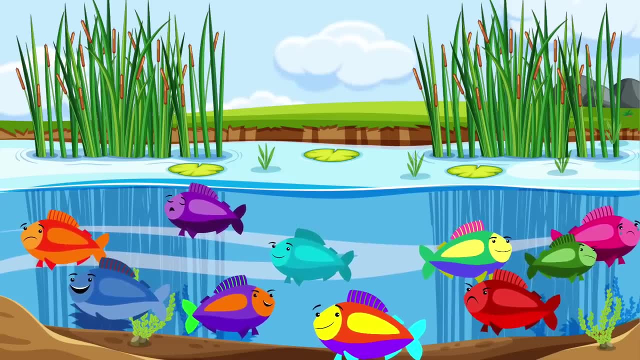 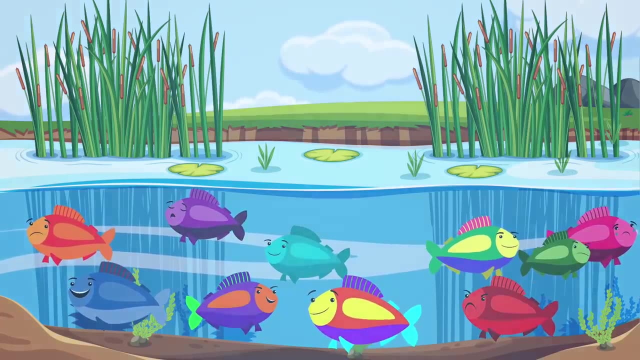 Zenden vemication. We might stop being the pond and find we've become one of the fish – like the angry fish, Something that hurts other people. But we're not the angry fish, We're the pond. Be the pond. Slowly we start to come back to the here and now. 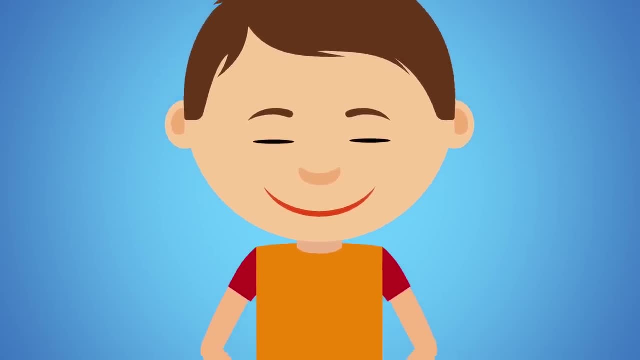 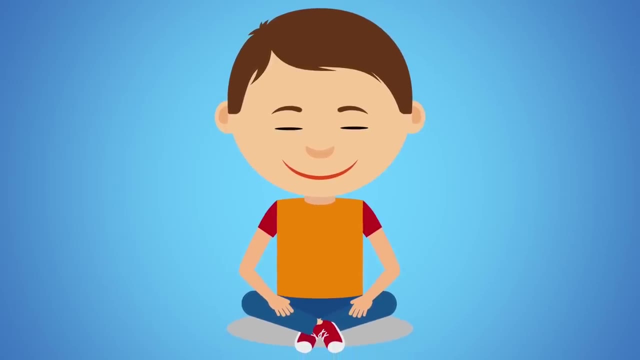 Isn't it interesting how many different kinds of fish we all have swimming around in our pond. So we practice just being the pond And when you feel like one of your fish has taken over, just say to yourself: Be the pond. This will help you come back to having all your feelings just swimming around, happily together. 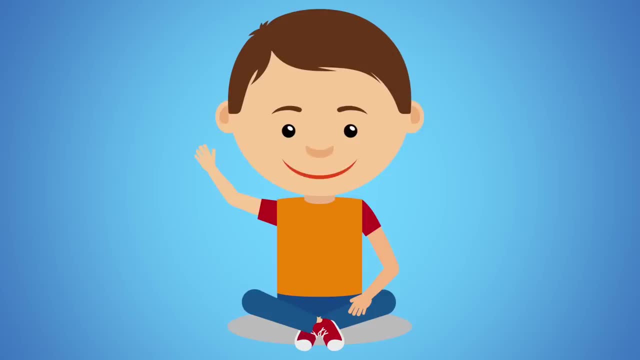 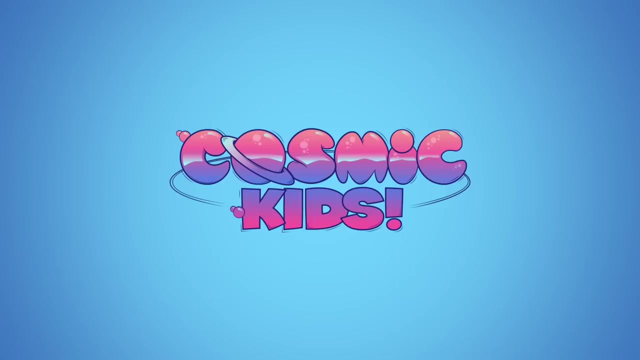 Thanks, Jack, for your help today And thank you for doing this Zen Den. You really are becoming a true Zen Den master each time you practice. I'll see you again soon for more Cosmic Kids, Yoga and Mindfulness. Bye, bye. Transcription by CastingWords. 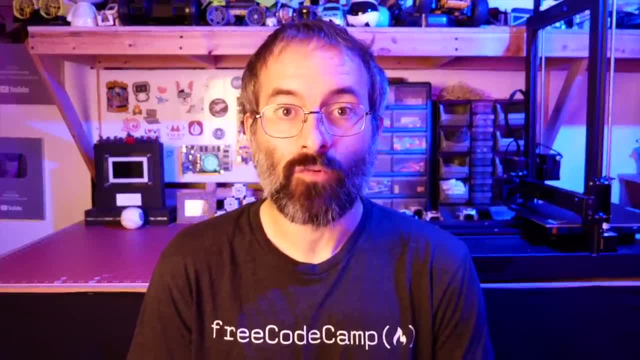 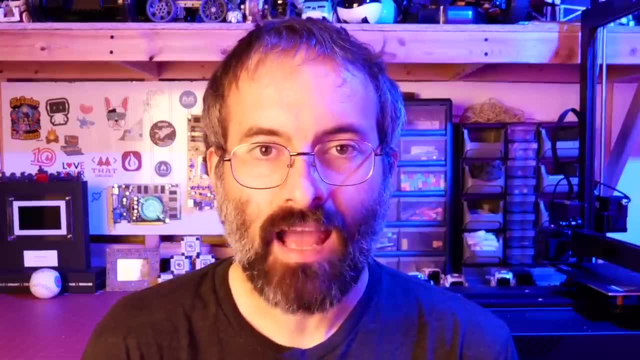 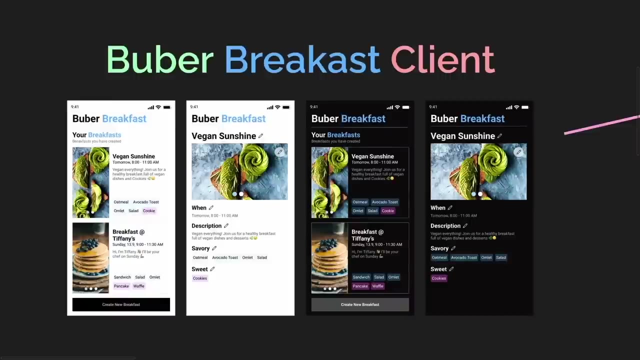 In this NET 6 course, Amakai will teach you how to build a REST API. Amakai is a software engineer at Microsoft and he is great at breaking down complex technical topics in a way that's easy for beginners to understand. Hi everyone, Today we're going to be building a CRUD-based REST API. 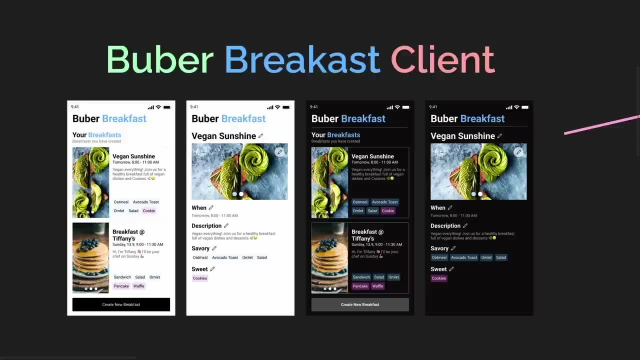 completely from scratch. I'm really excited to be collaborating with FreeCodeCamp on this video, so I really hope you're going to like it and I can't wait to hear what you think. Okay, so what are we building today? Well, today we're going to be building the backend. 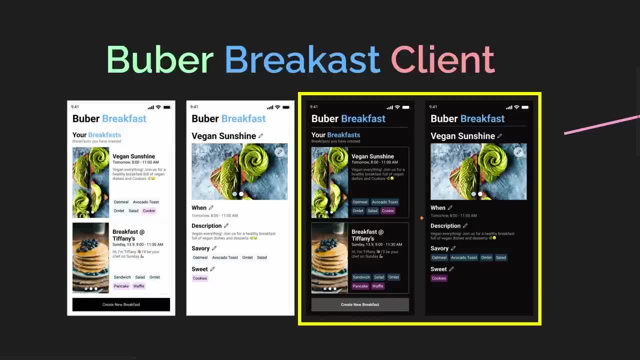 for the fictional application Boober Breakfast. And now, what is this Boober Breakfast application? Well, it's basically a system in which you can create breakfast And, as you can see, every breakfast has a title, a description, a start and end time. 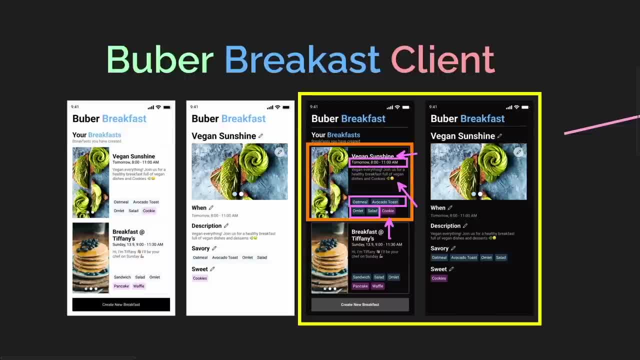 some savory items over here and also some sweet items, And because what we're building is a CRUD-based REST API, then, as you would expect, the actions that we can do are create the breakfast that we will be including in the breakfast. So just let me know in the